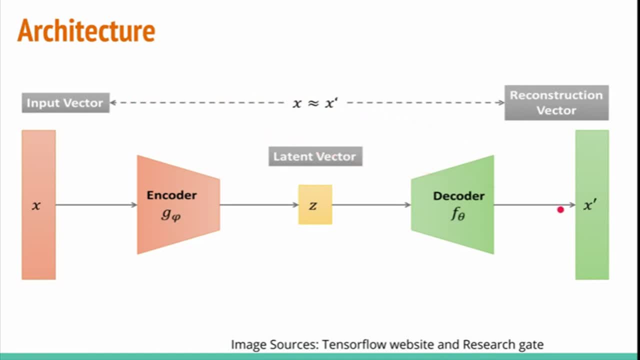 of autoencoder is the output. x bar is constrained compared to the x. Now I will talk about it as I go into the detail. Let's first understand an autoencoder architecture to understand what the output of autoencoder will be. Now, an autoencoder can be divided into two parts. One is the encoder. 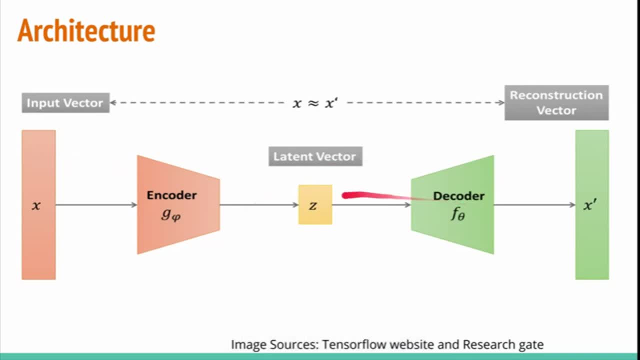 over here. and second is the decoder. Now the encoder is mapping from input space x, into a lower dimension latent space, and this z is the lower dimension space and it's called also called the bottleneck layer. So basically, you have an input, you have a bottleneck layer over here. 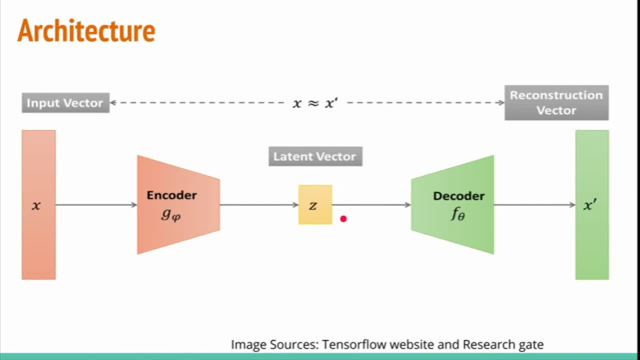 And this is a lower dimension space. Now, at this stage, it is nothing but lower dimension representation of the data and it's completely in an unsupervised manner. So autoencoders are unsupervised learning technique. You don't need a label data. 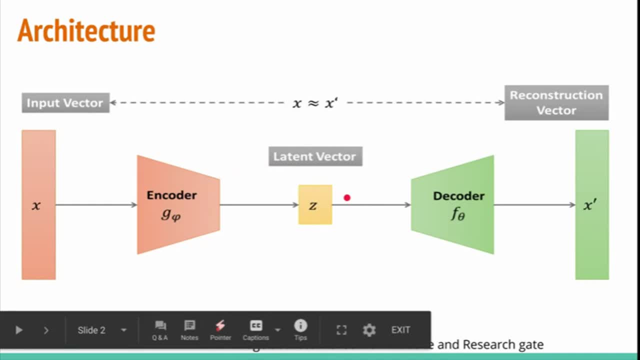 Now what it does over here is nothing but a dimensionality reduction as to what a simple PCA does. But the potential benefit of autoencoder here is how they treat non-linearity in the data. So basically, it allows model to learn very powerful generalization compared to your PCA. 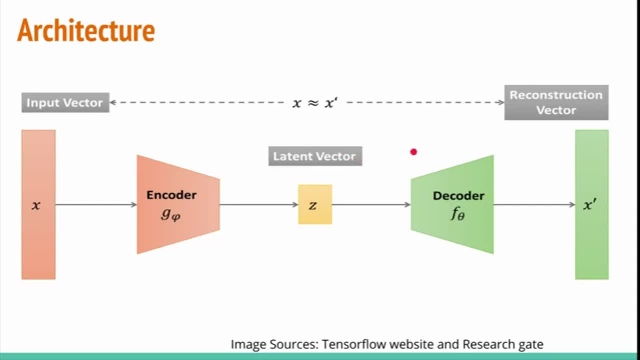 and it can reconstruct back the output with significantly lower loss of information than PCA in a non-linear space. So that's the advantage of autoencoder over PCA. Your PCA is completely on a linear data set and here it's going to be on a non-linear data space. 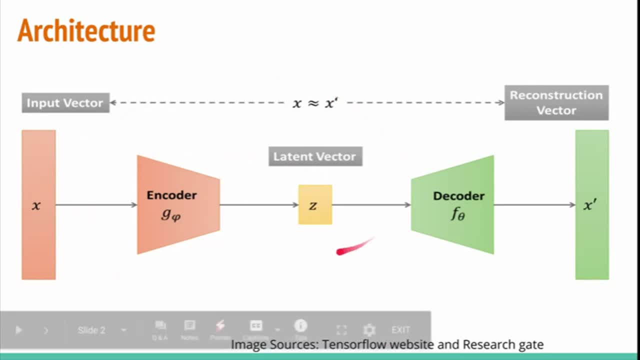 Now that's about encoder. So encoder takes an input x and convert into a lower dimension space And this space can be directly used for your dimensionality reduction and you can directly feed it into your model. And if you want to reconstruct the space, that's where the decoder 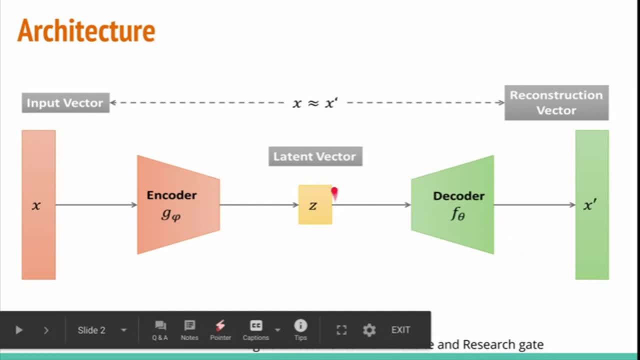 comes into play. So the decoder is nothing, but it takes the data from the lower dimension latent space into a reconstruction space where the dimensionality of the output x bar is equal to the output x. So now, if you see, x bar is equal to x, but if you think like a compression, right. 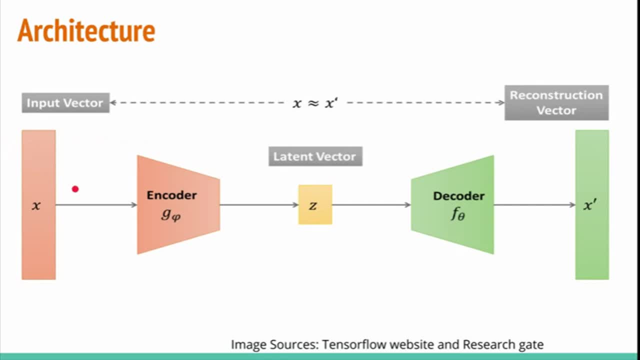 so what it do is: if you take an image, you compress the image, you compress the image, you compress the image and you uncompress it. you typically have lossless compression, right, You get the image as it is. But in case of an autoencoder it is basically a lossy compression, So it compresses. 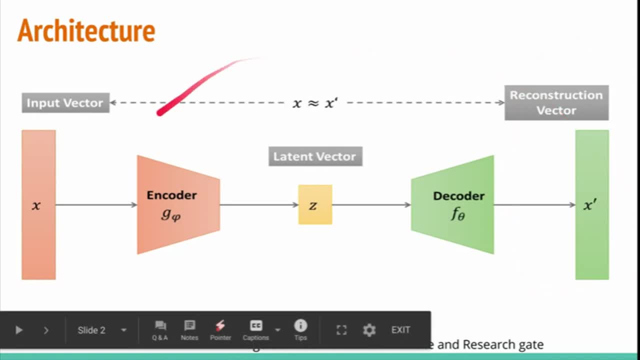 and uncompresses. and when it uncompresses it it tries to be close to the input, but not exactly close. That's the difference between, like, a typical lossy algorithm and a lossless algorithm, right? So, basically, your autoencoder can also be used in an image compression. So, if you want to, 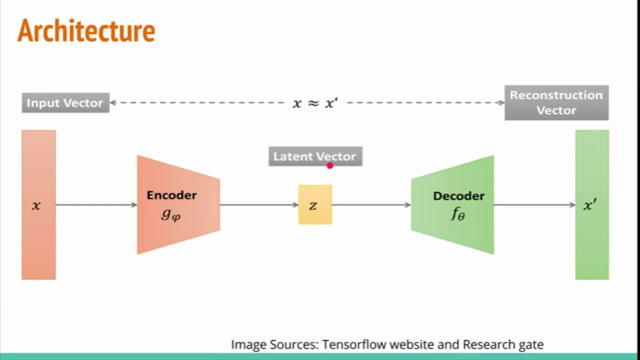 have an image, compression techniques and everything, but you will have a lossless compression over, So a lossy compression over that. In this case, the difference between the output representation and the input representation is called the reconstruction error. Basically, the error between your input vector and output vector, that's called the reconstruction error. 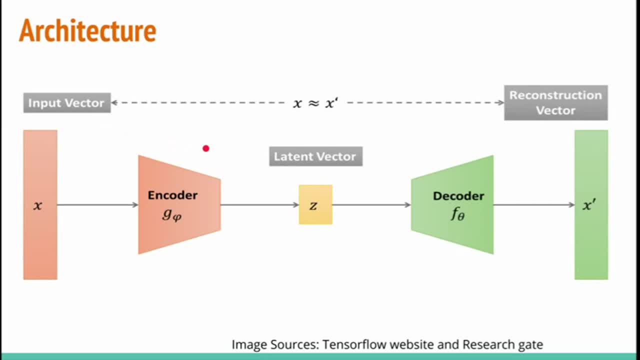 One potential use case of autoencoder is anomaly detection. While there are plenty of use case of autoencoder, there are predominant use case, that is, that we can think of as anomaly detection. And the reconstruction error that we are talking about between the output to the input is what we use to detect whether an input is anomaly or not. 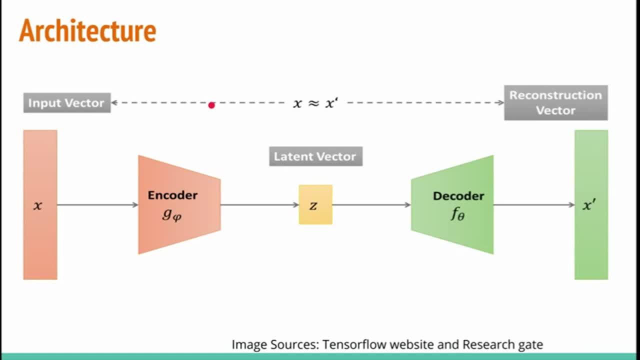 I'm going to more focus on anomaly detection here on. So think about cases where your IoT sensors or missions, or even your sensors in your CPU and memory devices- Typically there is one in a million possibility- a lot of cases in this missionary and IoT sensor to fail. 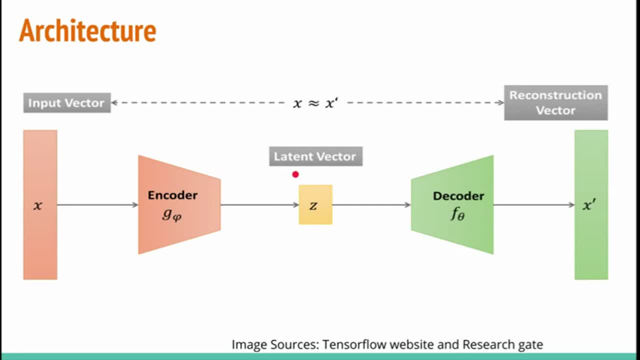 You will not have a lot of negative instances- Your data is completely imbalanced- but you will have a lot of positive instances And it's very difficult to basically train a model with such high imbalance, And that's where autoencoders are pretty much superior modeling technique in these. 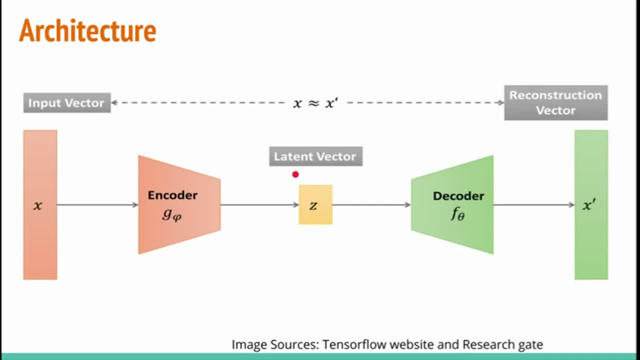 cases where you have very low 0.001% of error samples, While it can be used with more like negative samples as well. That's also quite possible where you don't have a lot of labels in that case. So sometimes it's very. 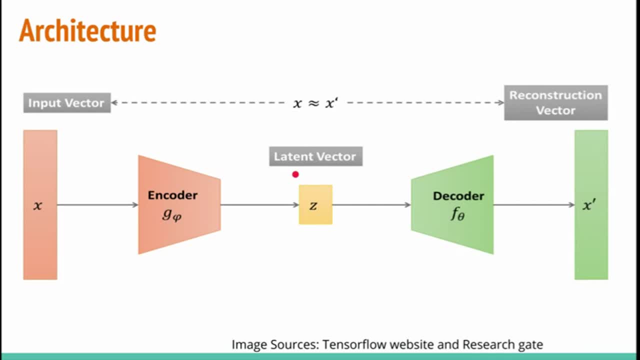 difficult labeling or very expensive labeling the data, but you know your normal behavior. So basically, what you can do is you can train your model with the normal data And then, when you're doing an inference or evaluation, you can see how the data performs against the abnormal data. So I'm going to explain that in detail. 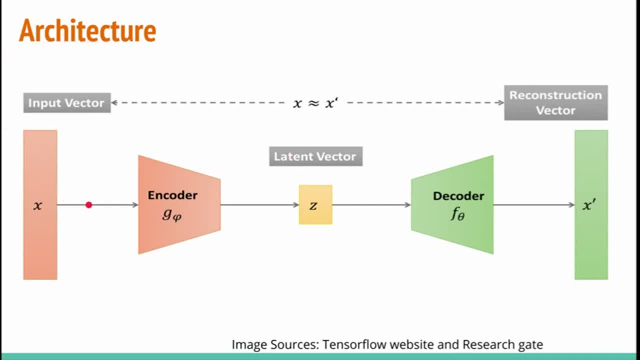 So what you do is you pass your autoencoder with the majority classes- all the normal data in the case. You will train your model only with the normal data or the majority classes. The training objective for the autoencoder in this case is to minimize the reconstruction error. We said. 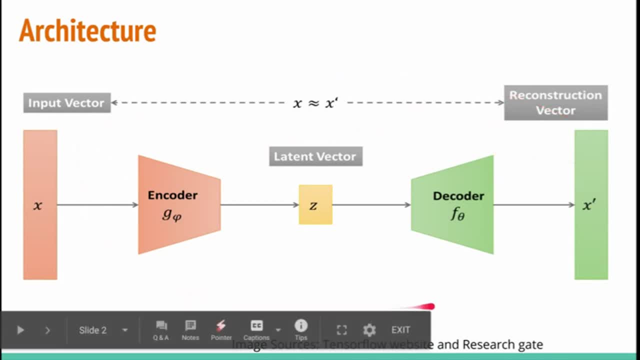 reconstruction error is the error between the output and input And the training objective of this autoencoder here is to minimize the reconstruction error over here. Now, as the training progresses, the model weights are updated over here, the encoder and decoder. The encoder is nothing but a downsampler and decoder is nothing but an upsampler. I'm going to 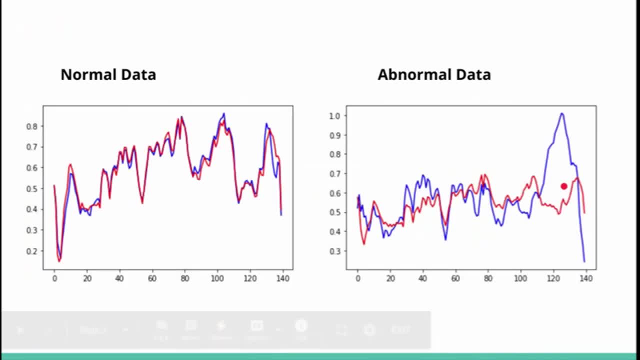 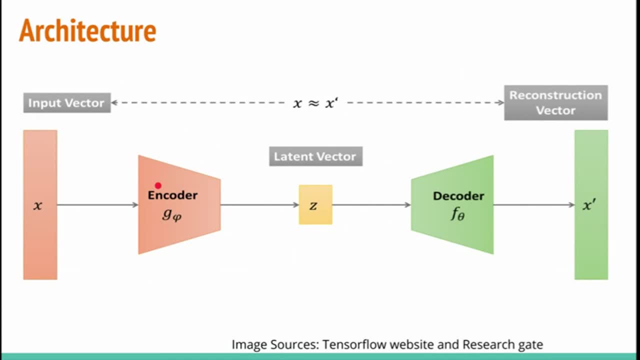 show some of the architecture examples And this encoder and decoder. I'm sorry, the encoder and decoder can be your typical feedforward neural network. It can be a convolution neural network or it can be an LSTM neural network. So as the training progresses, the model weights are updated. 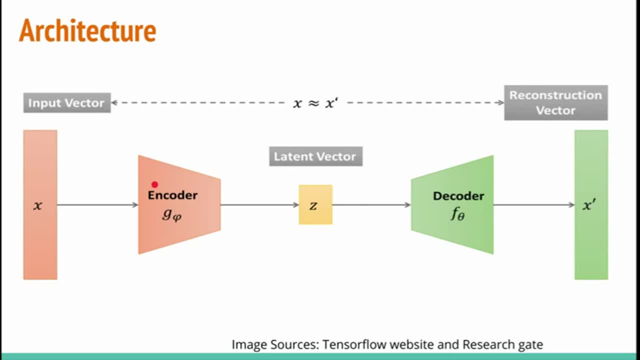 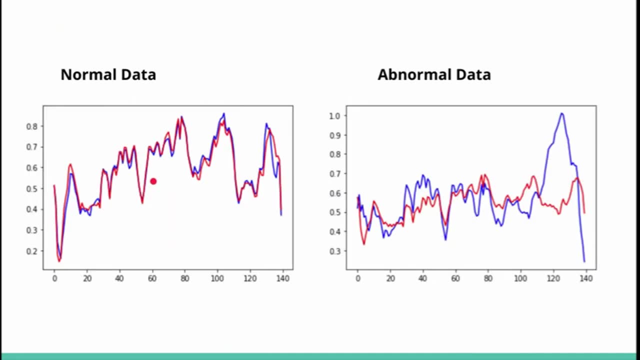 to minimize the difference between the encoder input and the encoder output. Now what the autoencoder does? it learns a reconstruction function that works well with normal data. Basically you get a low reconstruction error and works poorly with an abnormal data. that that is going to be a minority. 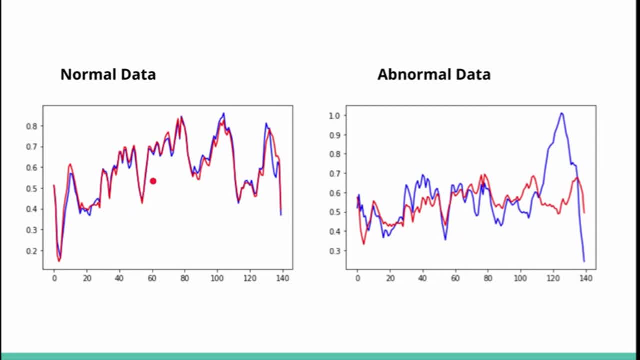 classes where the reconstruction error is pretty high And we can use this reconstruction error for anomaly detection. So this is an example of an output from a trained model And if you see, the model was trained using the normal data and you can see the blue line is the actual data. 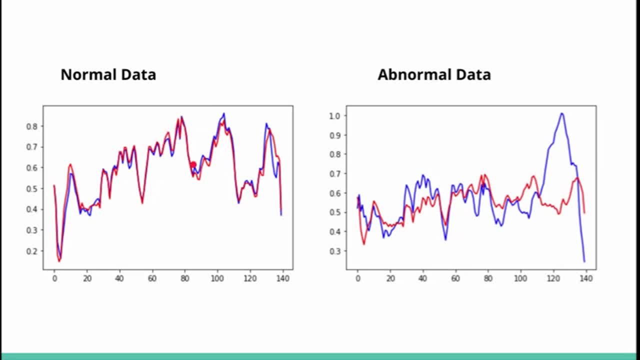 whereas the red line is the output of the model. that is a reconstructed output And you can see. basically, the model performs well on a data and the reconstruction error is the difference between the blue line and red line. this is the reconstruction error. now, what you do over here when you 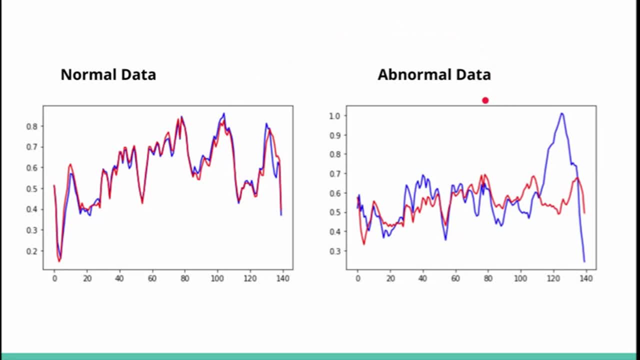 pass an abnormal data. the model has not seen the abnormal data right. if you see over here, it is not fitting correctly. the reconstruction error is pretty high. there's a sudden peak, there are lows and sudden high peaks and everything right. so the model will not fit perfectly and there will be a high. 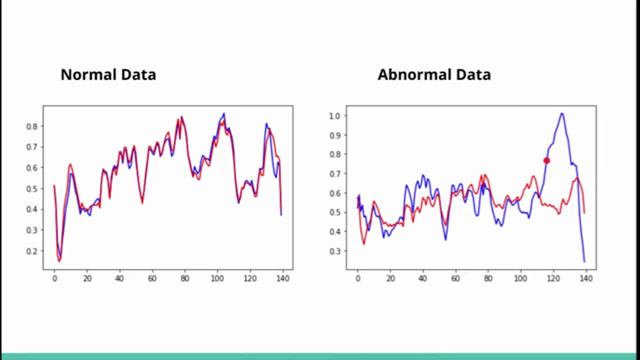 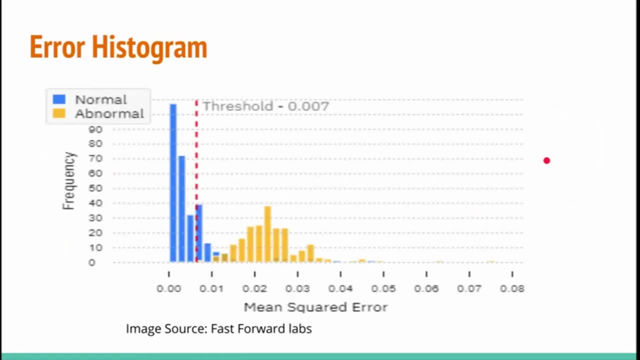 reconstruction error and this reconstruction error is what you are going to set a threshold and then identify whether it's a normal data or anomaly data. so if you see this slide here, the distribution of your errors for normal sample is very small. the blue one is the normal sample. the distribution of 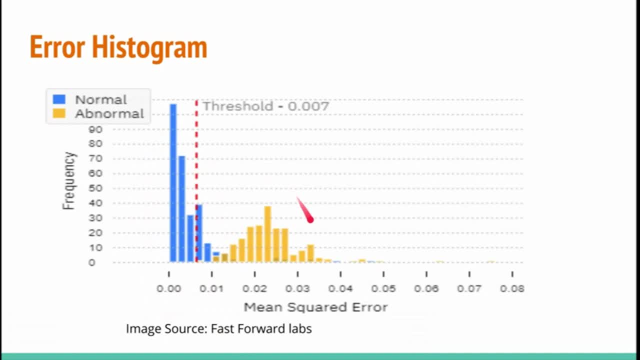 this mean squared error is very small, whereas for your abnormal data is higher than the normal data. so when you are training an autoencoder right, it's going to separate out your normal and abnormal classes. basically, you can now slightly little label data so that you can evaluate your model right, but you can also use in the training validation you. 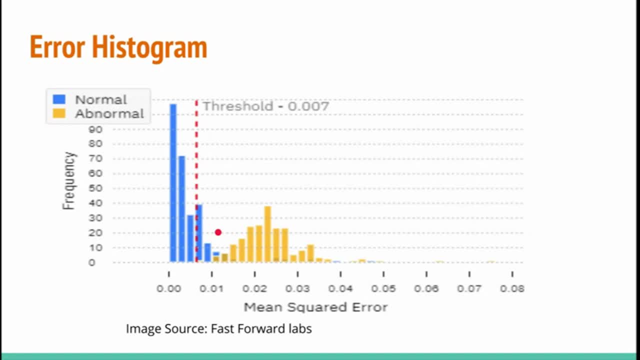 can both use your trained data and your abnormal data and then see how the model performs now. this is how it looks like right now. what you do is you take the mean of your- in this case, the mean of your normal data and put one or two standard deviation, or even three standard deviation, depending on your 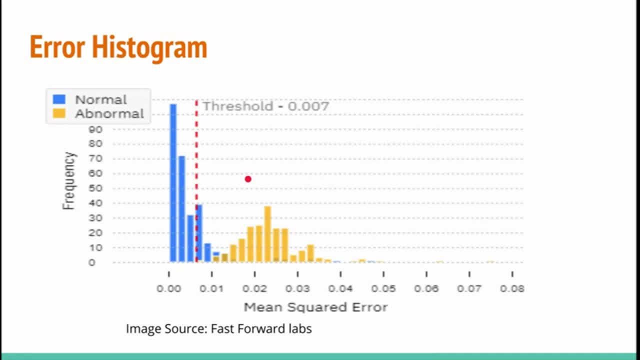 business use case as a threshold and when you feed in new data in real time. and spice results means that if the, if the incoming data is above the threshold, then it's an anomaly. if it is less than the threshold, then it's a normal data. so that's so basically, you you train a neural network model for train a auto. 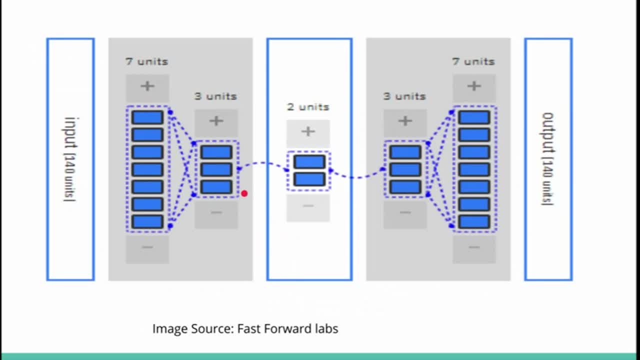 encoder model for anomaly detection. now, as I said, your anomaly detection can be a feed-forward neural network. if you see your input data with 140 variables right and you have a known sampling, you have a 7 unit or feed-forward neural network. then you have a 3 unit or수�ssa. 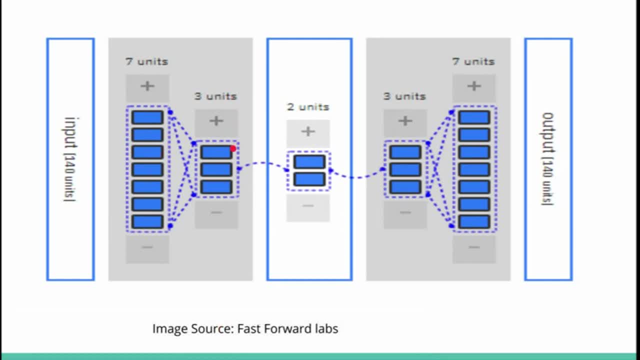 household data with defaulting result which is 10000 capital margin. so all that is a well-designed applicationçi. there's a different platform. you can find it these days, right? I use the key function to compute performance analysis. I use the key function to compute performance analysis. 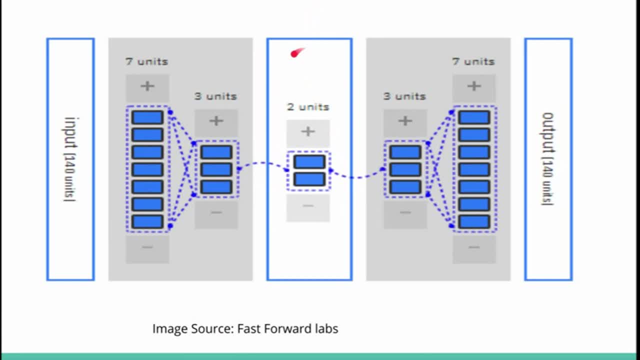 and then you have a two unit bottleneck layer, which can be your basically dimensionality reduction layer as well, and then what you do is, again you have upsampling of the same size. so basically, you have three units, seven units, and the output layer, which is similar to the input. 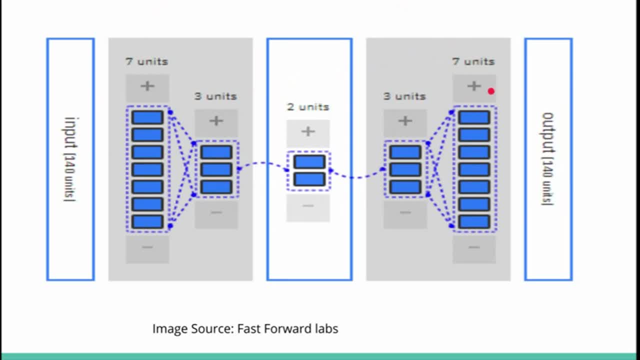 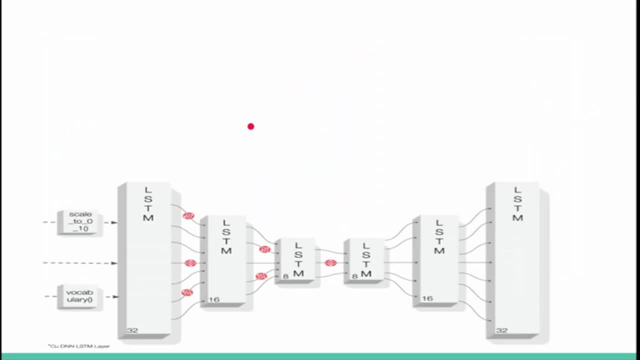 layer and, as i said, it's a lossy compression kind of. if you can correlate, it's kind of a lossy compression, so you'll have an reconstruction error that is between the output and input. or it can be a convolution neural network, where you take a image and then you reconstruct an. 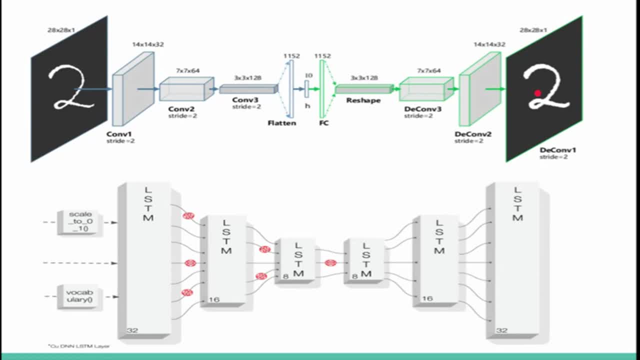 image. the image will not be perfect. there are some cases where image where you can denoise a image. basically, if you are noisy image, you have denoising auto encoders which can denoise a image and then you have an lstm and typically it's used for time series models where you want.